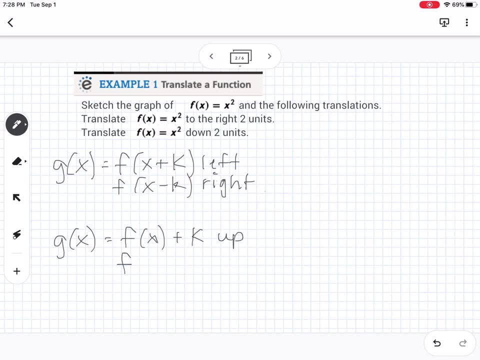 be up and f of x minus k is going to be down. So those follow the rules of what we think. Okay, so now if we go to our graph, there's a couple different ways we can do this, So we've talked about with the previous lesson. you can type stuff into Desmos. you can type: 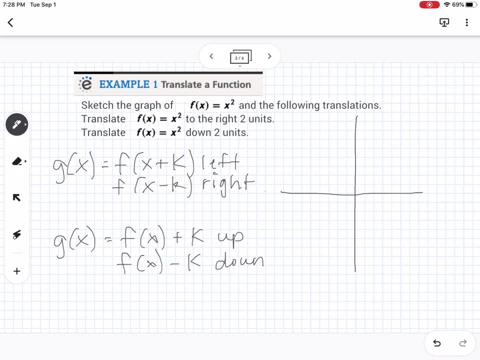 it into your graphing calculator. You're not expected to just get an equation and know exactly what the graph looks like. It's totally fine to graph it on technology, or you can make a table to figure out what the graph's going to look like. 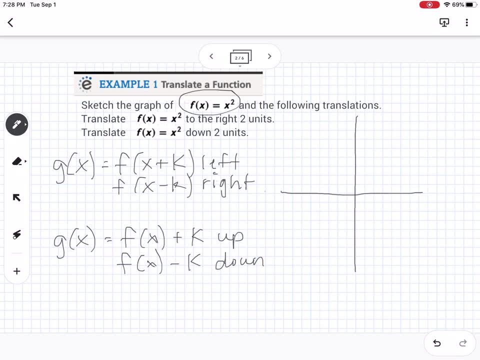 So if I'm starting with the graph of f, of x equals x squared, let's just say I'm not sure and I'm going to make a table. So if I plug in 0, I know that 0 squared is 0.. 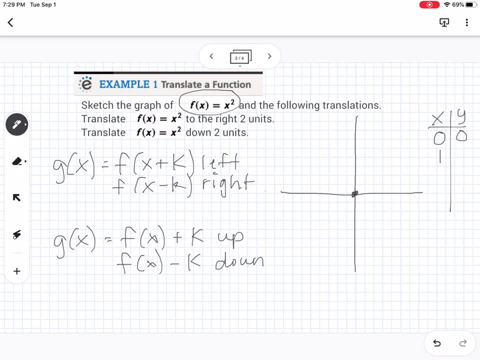 So 0, 0 is going to be on my graph. I know that 1 squared is 1, and I know that negative 1 squared is also 1.. So those two points are going to be on my graph. I know that 2 squared is 4, and negative 2 squared is also 4.. 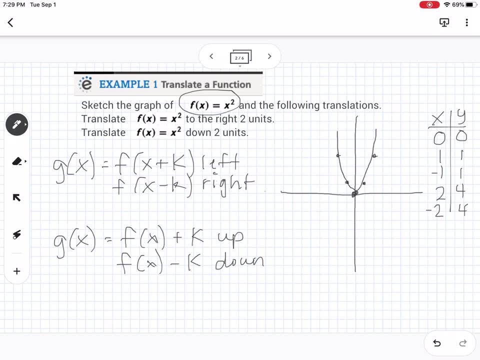 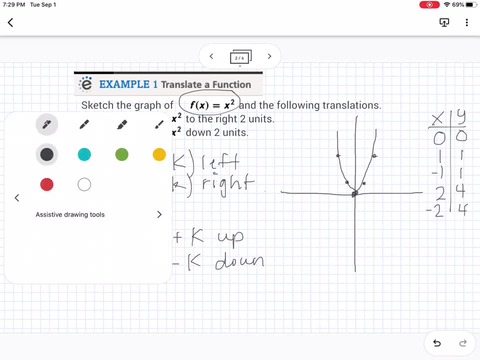 So right there, there's my f of x equals x squared graph. Okay, now I want to sketch, So let's change colors here. So I'm going to use, I'm going to use green, We're going to sketch the translation to the right two units. 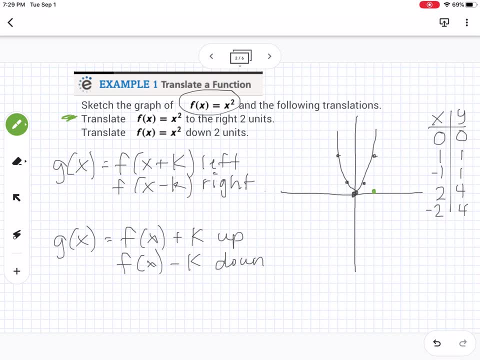 So that means that we're going to go right here, but it's going to be the same graph, so it's going to look something like that. So this graph- let's see if I can come right up here- So this is going to be- let's call this g of x. 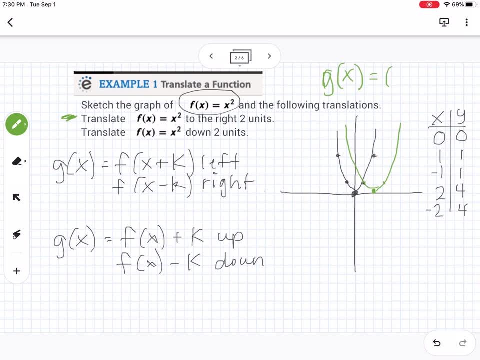 would be so, since it's a left and right shift, it'd be inside the parentheses with the x, and since it's to the right, it's going to be minus 2 squared. So that's what my function would be. So I'm going to use a different color here. 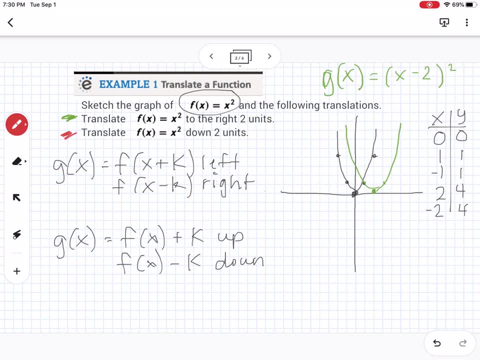 Let's use red. So now I want to shift it down two units, So let's go right here. So there's my graph. Again, these graphs aren't perfect, but there is my graph, So I'm going to use the graph shifted down two units. 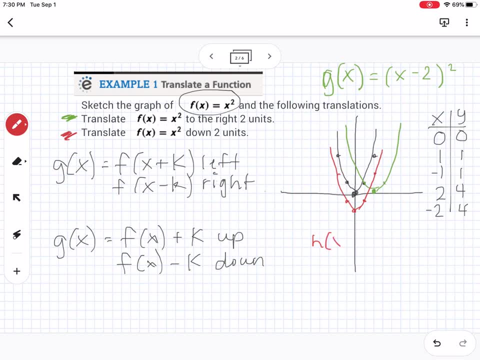 So this would be- let's call this h of x. This would be x squared minus 2.. So you can notice the difference between the green equation and the red equation. One- the 2- is inside the parentheses with the x and one it's not. 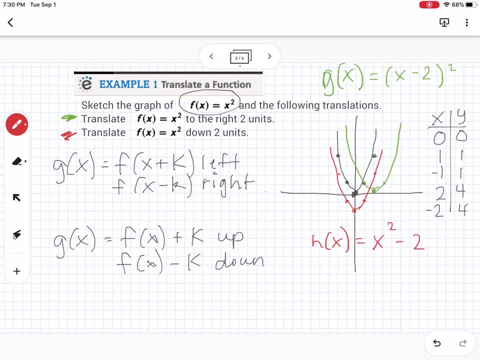 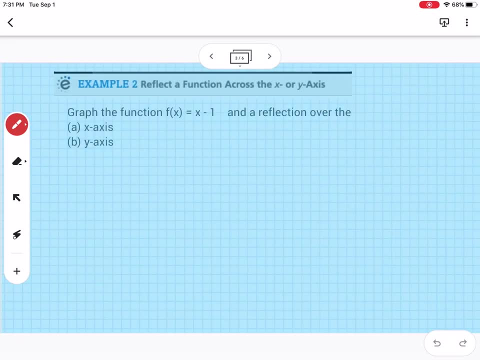 So if you're moving it left and right, it's inside the parentheses, If you're moving it up and down, it's outside. Okay, so that is translations. Okay, so example 2 is reflections. So we're going to graph: the function f of x equals x minus 1. 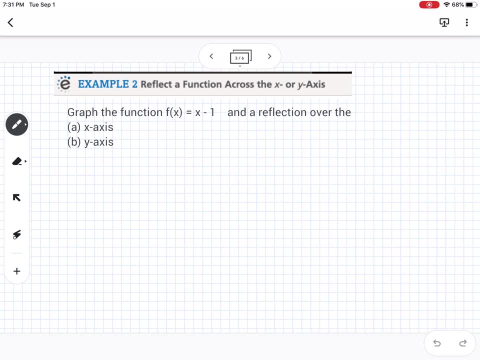 and a reflection over the x-axis and over the y-axis. Okay, so first of all, let's talk about what reflections look like with the equation. So if you have the negative on the outside, that is a reflection over the x-axis. 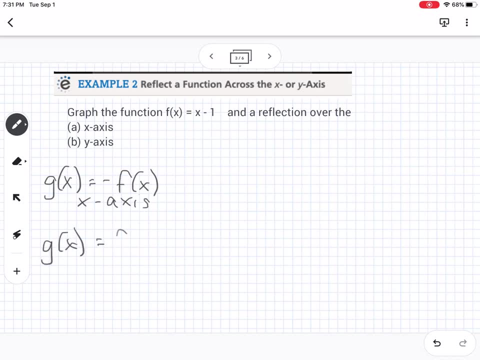 Okay, And if you have the reflection on the inside, that is the reflection over the y-axis, So where the negative is tells you what type of reflection you're talking about here. Okay, so we're going to graph. f of x equals x minus 1.. 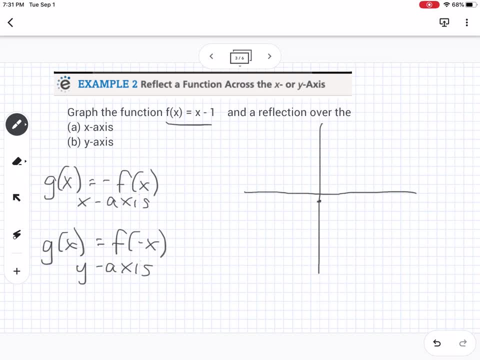 So my y intercepts at negative 1, and my slope is going up 1 over 1.. So we can sketch in. There's my original f of x. Okay, so then let's talk about. let's go to a green. 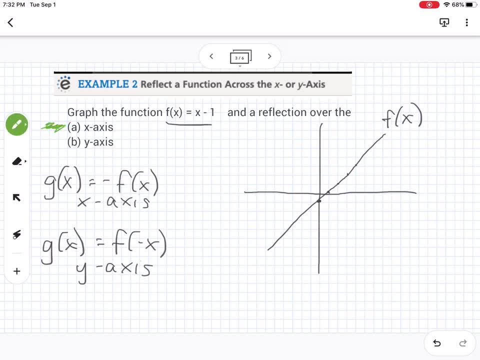 and we're going to use that to talk about reflection over the x-axis. So over the x-axis means that it's going to be a negative on the outside. So I'm actually going to write this first. So let's say it's g of x. 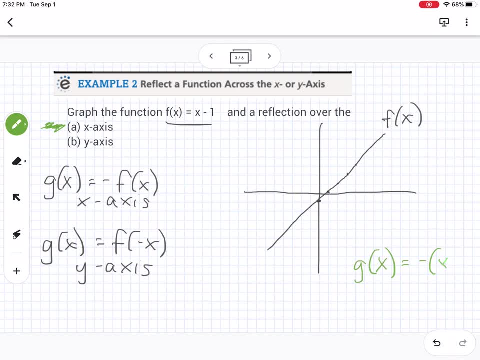 It's going to be negative x minus 1.. So we can visually see what that's going to do to our graph. So this point here is going to stay at 0, where this point's going to reflect over here. This point's going to reflect down here. 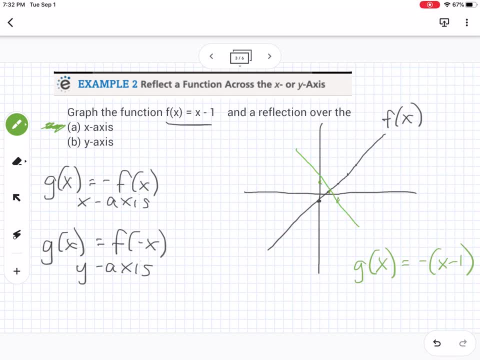 And we can sketch in what our graph's going to look like right there. Okay, And then if we distribute this x, let's figure out: so this is going to be negative x and then negative negative 1, so it would be plus 1.. 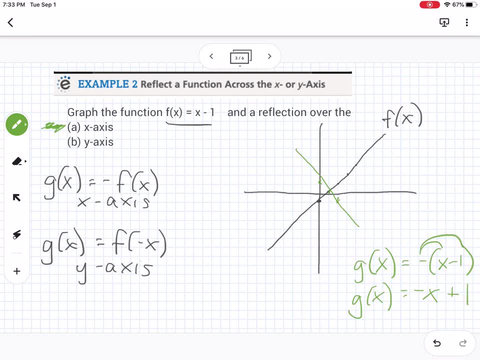 So then, if we look at that graph- even though my graph is not perfect- we can see we should have a y-intercept at positive 1 and a slope of negative 1x. So that matches what we have. Okay, so now let's change our color here. 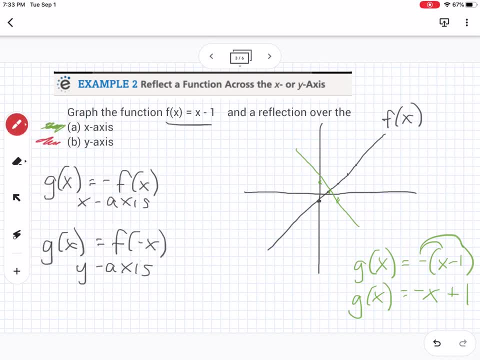 So now we're going to look over the y-axis So again we can reflect. So we know that point's going to go there, This point's going to stay at 0.. This point is going to see. that point's going to be right there. 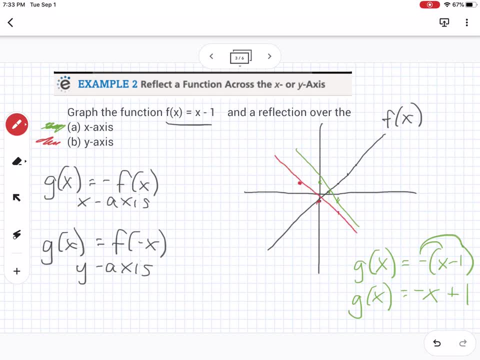 And we can sketch in that point that line. So then if I write this over here, so let's call this: h. This negative is inside with the x values. That means it's going to be negative x minus 1.. So if we simplify that, 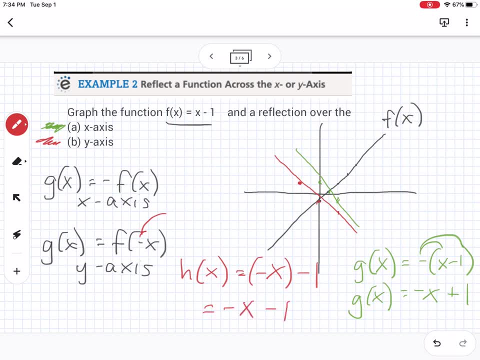 that would just be negative x minus 1.. So you can see that's going to be negative x minus 1.. And then we're going to get our y-intercept at negative 1. So we're going to be able to see that point. 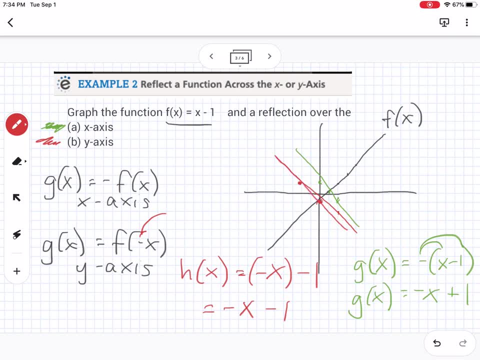 Other than the fact that my graph is bad. okay, our y-intercept's at negative 1, and our graph should be more closely going through that point right there. Okay, so that is how we have a reflection over the x-axis versus a reflection over the y-axis. 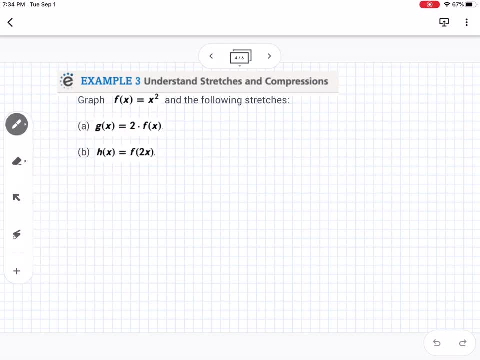 Okay, Okay. so our example 3 is understanding stretches and compressions. So, before I explain this, what I need you to understand is that, technically, a vertical stretch would be the same as a horizontal compression And a horizontal stretch would be the same as a vertical compression. 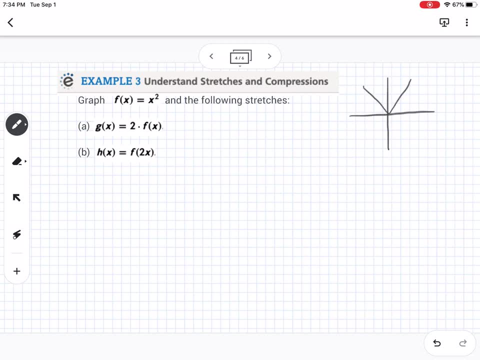 So if we're thinking of something- I'm just going to draw a picture up here- if you were to stretch it this way, it's going to make it narrower, which is compressing it this way. So when we're talking about this, 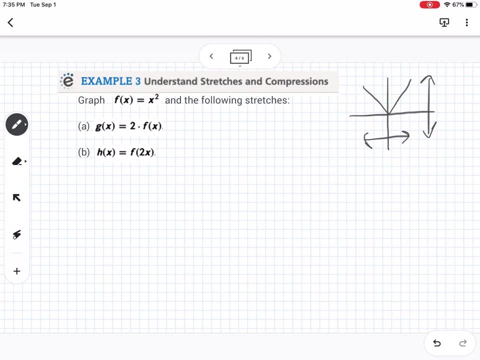 the number's in a different place, but the graph might look different. It might look the same, Okay. So, for example, let's say, if we have an, a value that's outside, so it's just a number out front of our function. 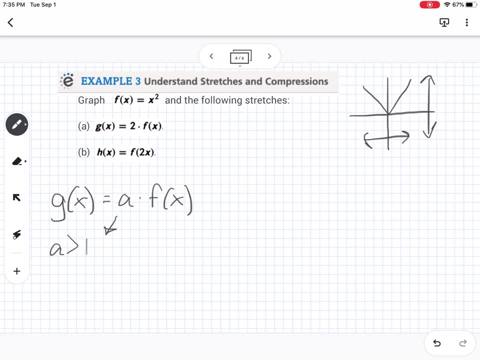 that a can be greater than 1, it's going to be a vertical stretch, and if it's between 0 and 1, it's going to be a vertical compression. Okay, And then we have, if the a is inside, with the function. 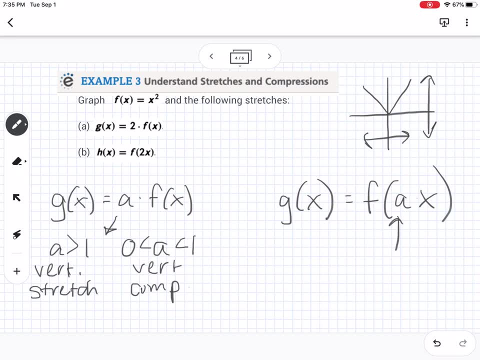 so this time we're going to talk about horizontal. So if this time, if a is greater than 1, it's a horizontal compression. So remember we talked about that. horizontal compression is going to look the same as a vertical stretch. Okay. 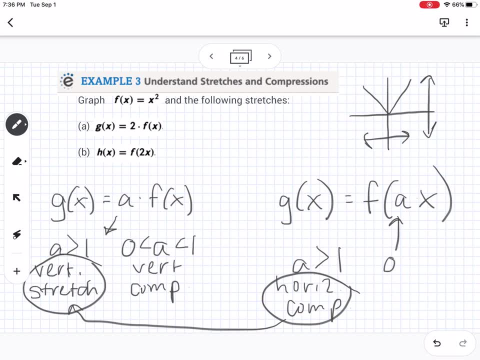 And then if it's between 0 and 1, it's going to be a horizontal stretch, Okay, So I'm going to take all of that and then we're going to sketch these examples here that we have. Okay, So we can actually 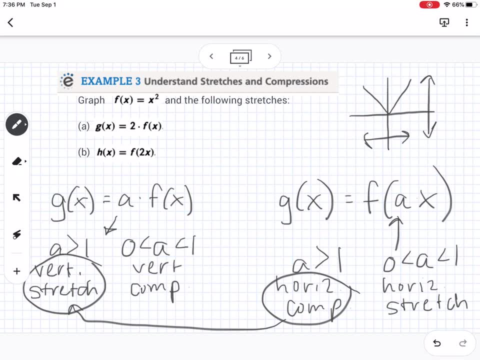 so this is one of those that you can see that the 2 out here is going to be a vertical stretch and the 2 in here is going to be, or is going to be, a horizontal compression. So these graphs are going to look the same. 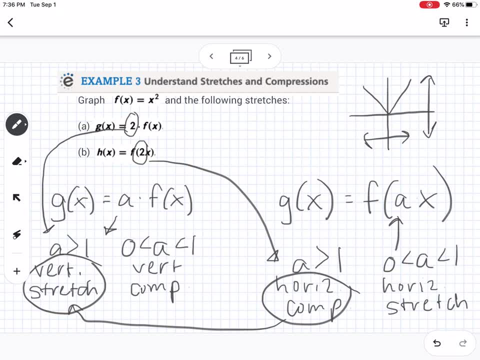 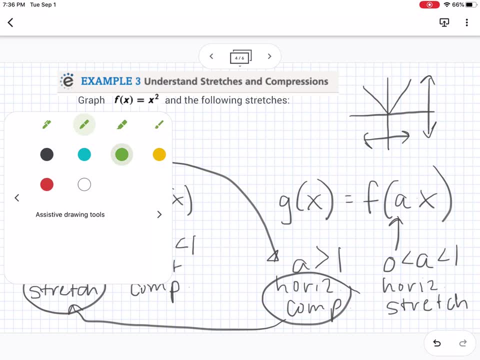 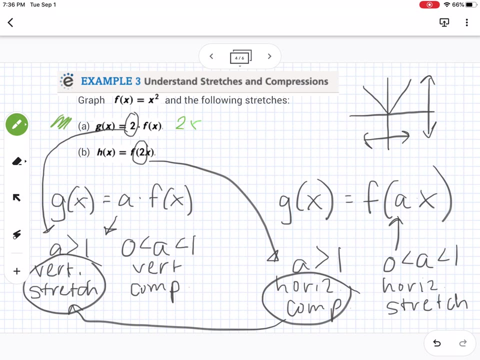 even though they're not exactly the same. Okay, So let's see here, Let's use a different color. Okay, we'll talk about this. So this would be. this would be 2x squared. that we're graphing. 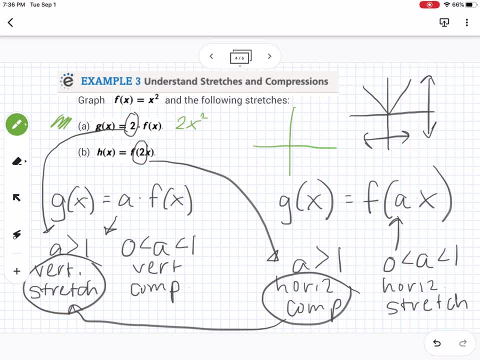 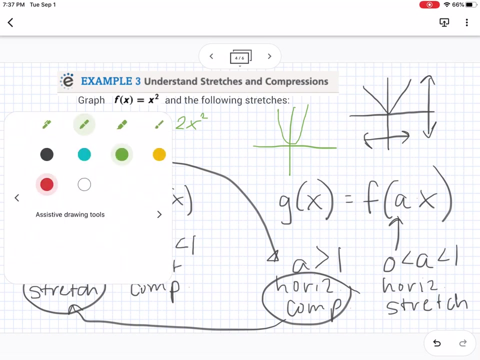 So that means, instead of being like having the point and it'd be, and because we're going to multiply every output by 2.. Okay, And then this one would be. this would be saying 2x squared. Well, we know, 2x squared is actually the same as saying 4x squared. 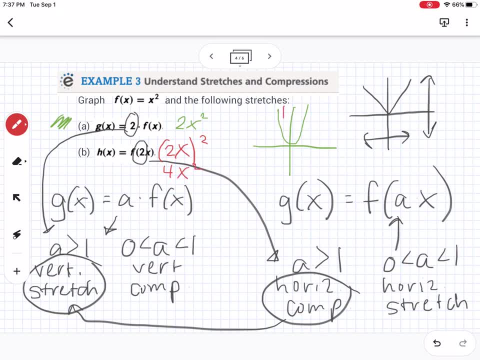 So it's also going to make it narrower, but it's going to make it even narrower than the green graph, So having the value placed differently. so it's going to do a similar thing as far as a stretch or compression, but it might not be equivalent. 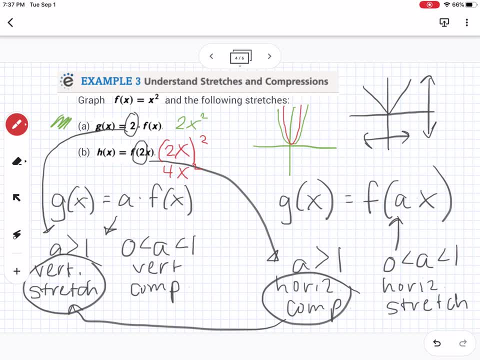 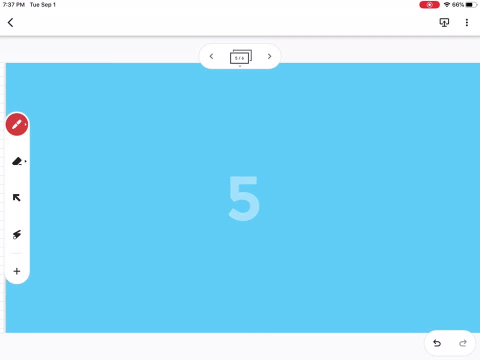 So having a 2 out front versus a 2 inside the parentheses could change it slightly. Okay, So that is that. So now we're going to talk about combining these together. So it's asking you to graph a combination of functions. 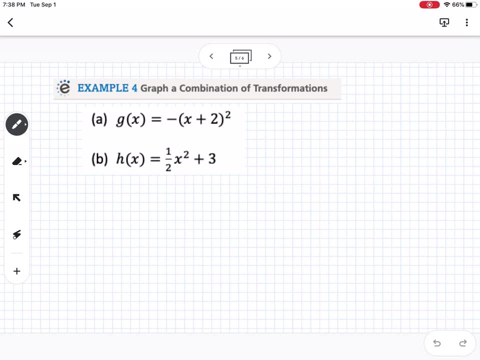 or right now. basically, what I want you to be able to do is describe the transformations. So on part we have a negative right here and that negative's out front. So we would say that is a reflection over the x-axis. Okay. 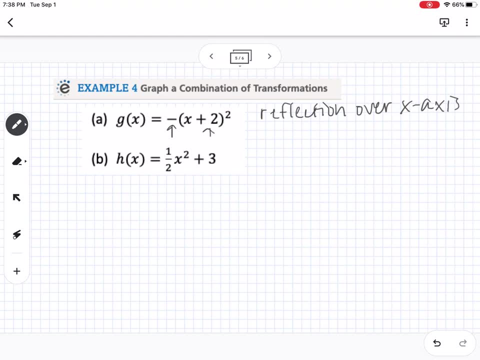 And then we also have a 2 inside. So that would tell us that we're shifting it left and right, and since it's plus, that means we're going to shift it to the left 2.. So those would be the two transformations for part. 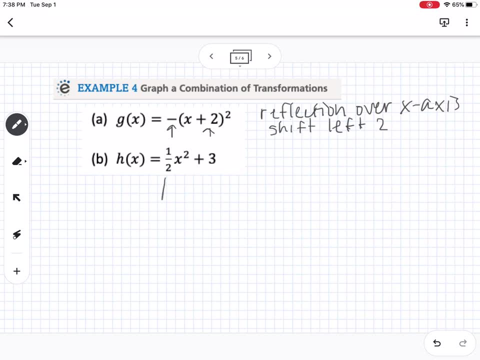 On part, we would say, okay, we have a 1 half and it's not inside the parentheses. So that means it's going to be either vertical stretch or compress, and we know 1 half is between 0 and 1.. 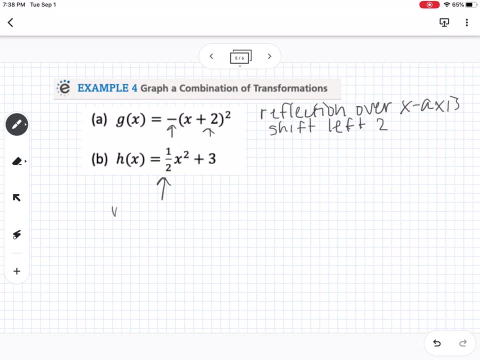 So that tells me it's going to be a vertical compression by 1 half and that plus 3, right, there is not inside parentheses also, so that means it's going to be shifting up or down. So that's going to be a shift up 3.. 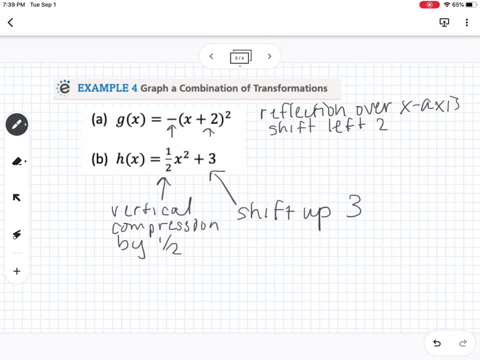 So we can have a combination of these, and this helps us to graph what the graph is going to look like. Okay, So one last thing before we're done with this, just a couple things. When you're doing the assignment, it might ask you to graph something. 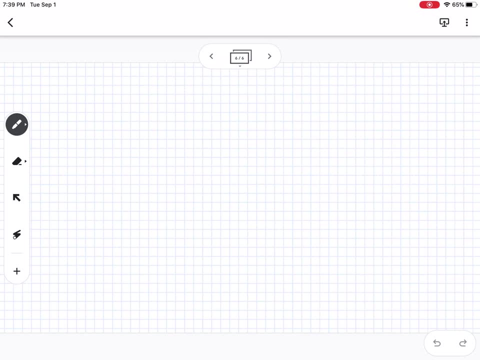 So I want to just real quick. let's say I have g of x equals the absolute value of x plus 3.. Okay, So some things about absolute value of x. So let's say I have g of x equals the absolute value of x. 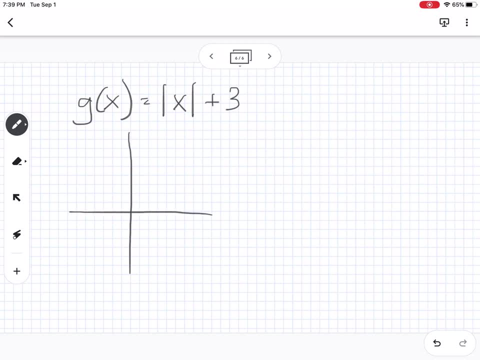 0 of x equals the absolute value of x. Let's say I have g of x equals the absolute value of x. 0 of x equals the absolute value of x. 0 of x equals the absolute value of x. Let's say I have g of x equals the absolute value of x.